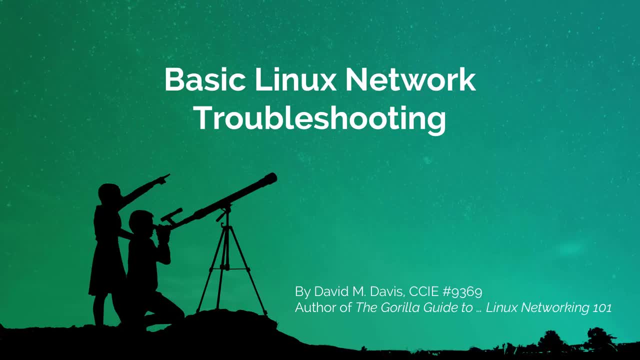 If you've ever tried to troubleshoot Linux networking, you might find out that it can be complex and it can be frustrating at times. But rest assured, you're in the right place. In this video, I'll walk you through some of the basics of troubleshooting a Linux network. 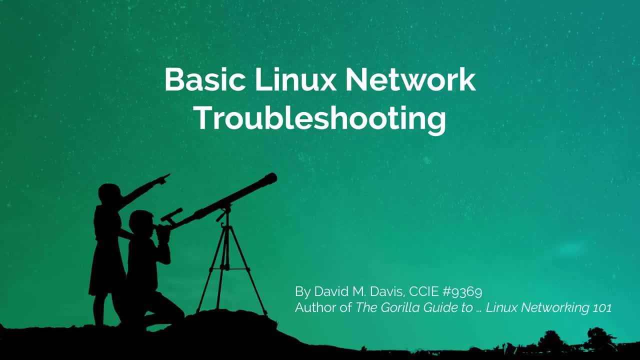 What I'll show you here are some of the steps that I went through in my book, The Guerrilla Guide to Linux Networking 101.. At the end of this video I'll show you how to download that book for free. so stay tuned. 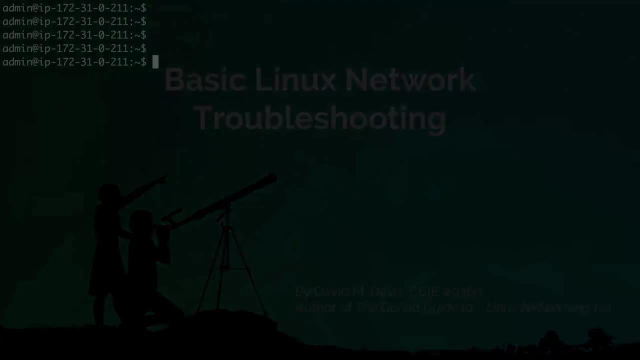 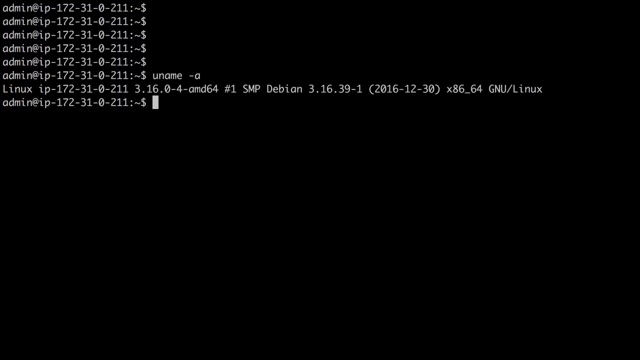 With that, let's jump over into Linux and get started. The first thing I do when I connect to a new Linux host that I'm unfamiliar with is I run the uname –a command. This tells me what version of Linux I'm on. In this case, it's a Debian Linux system. 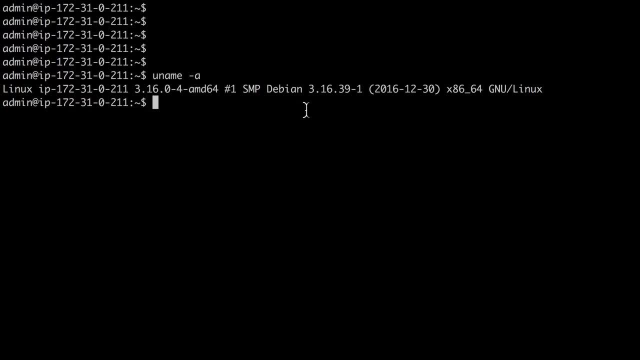 And that's important because the commands used and the syntax used can vary greatly from one Linux distribution to another. Now, in my previous video on Linux networking interfaces, I went through a couple of basic Linux networking commands which I think are worth reviewing quickly again. 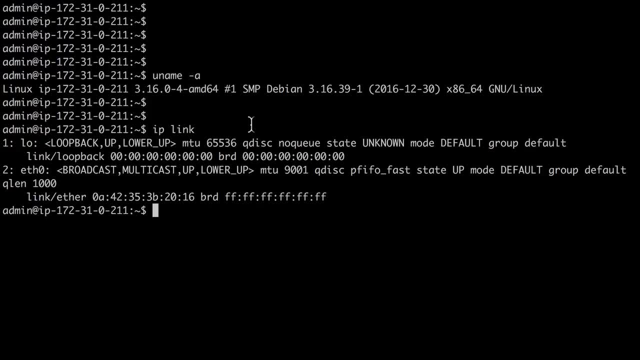 The first one was the ip link command. This command shows you the network links on your system and the status of those links. So, for example, here we have the Ethernet 0 interface. We can see that it is up, and the lower interface is up as well. 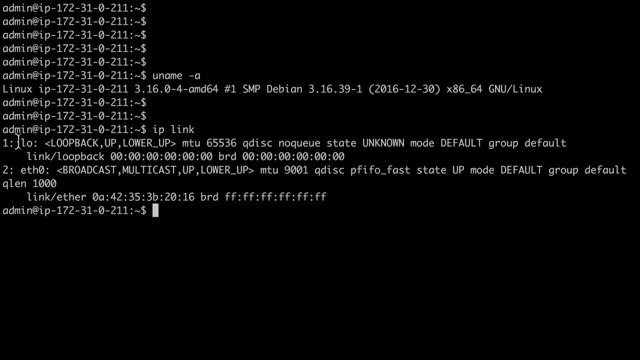 So the physical connection. We also see we have a loopback interface which is used to identify the system. You can learn more about the ip link command with the man ip link command. Another important network troubleshooting command is ip addr or ip address. 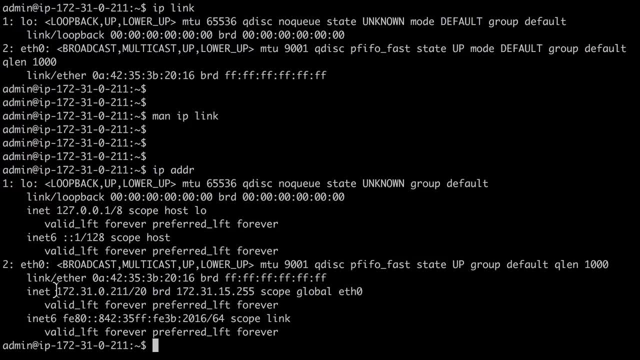 And this shows the IP addressing on the system. For example, the Ethernet 0 interface has this IP address assigned to it. You'll want to make sure that your system has an IP address. Any part of troubleshooting the Linux network should start off with ensuring 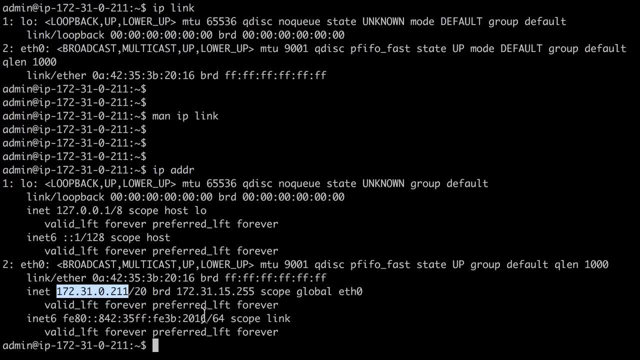 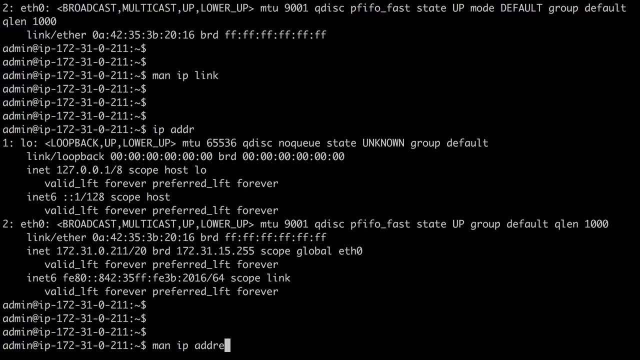 that you have an IP address configured and that your interfaces are up. To learn more about the IP address command, you can do man ip address. The IP address command is used not just to show the status or show the IP addresses that are configured. 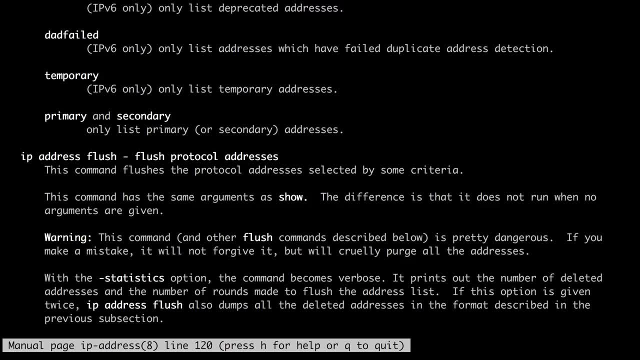 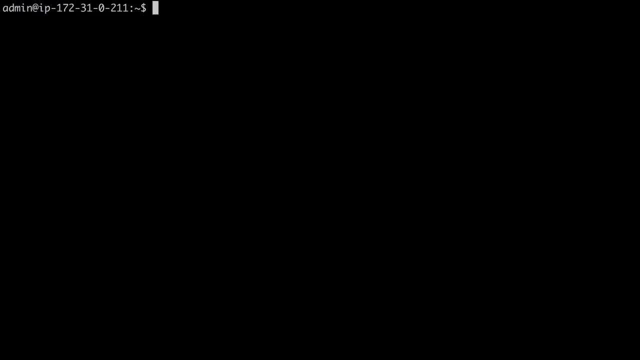 but also to reconfigure the IP addresses on those network interfaces. Now in this short video I don't have time to go into things like advanced network troubleshooting, subnet masking, routing tables and so on, But I want to point out a few basic Linux networking commands that everyone should be aware of. 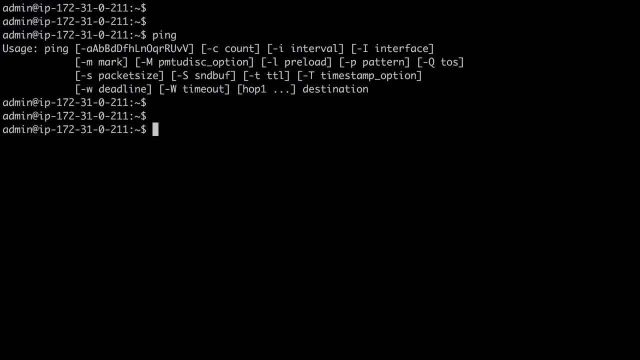 The first one is the ping command. The ping command is used to test network reachability. So, for example, let's say I do ping minus c5 to do a count of 5 pings And I ping the IP address 8.8.8.8.. 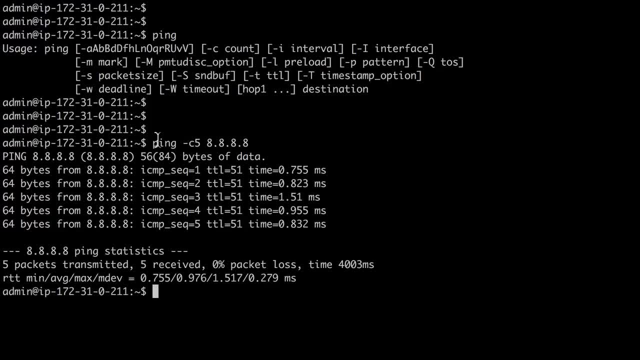 In this case we're going to send out 5 pings And we need to specify that in Linux because, unlike in Windows, where the ping command will stop after a certain number of pings, in Linux the ping command will go on forever unless you specify the number of pings or you press control c. 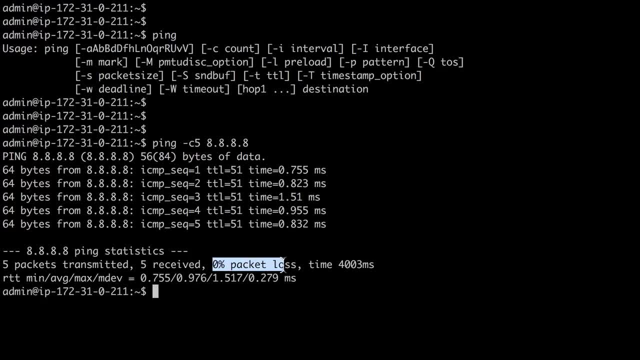 Now, in the case of this ping, we had 0% packet loss, So we had 100% reachability. That's very good, And we also had an average round-trip time of 0.976 milliseconds. That's very, very fast. 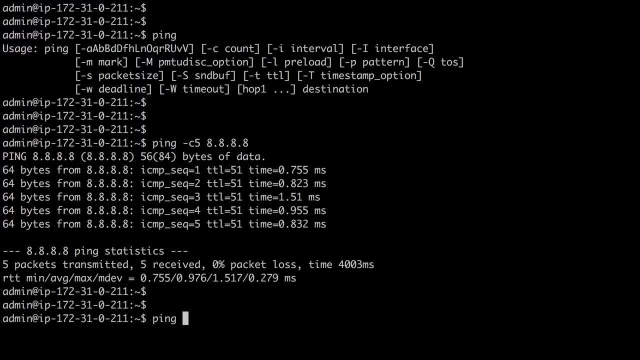 So we've got great network reachability to that IP address. If we try another one, this time to the 1.1.1.1 IP address, let's see what happens in this case. Uh-oh, It looks like this time we had 100% packet loss. 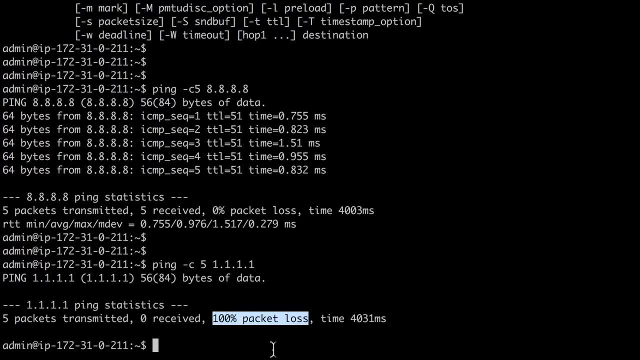 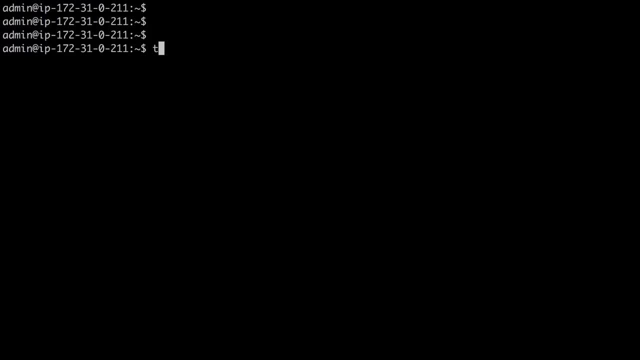 So 0 reachability And it looks like we cannot communicate with that IP address. Another tried and true command for network reachability is traceroute. In Linux that command is one word, traceroute- And let's do it to the same IP address. 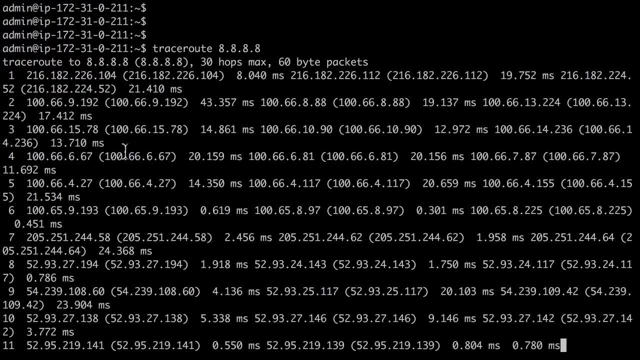 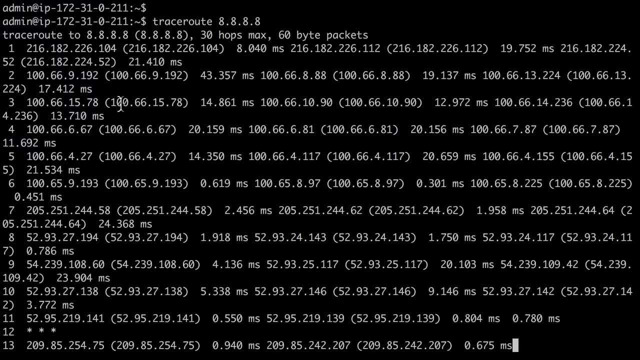 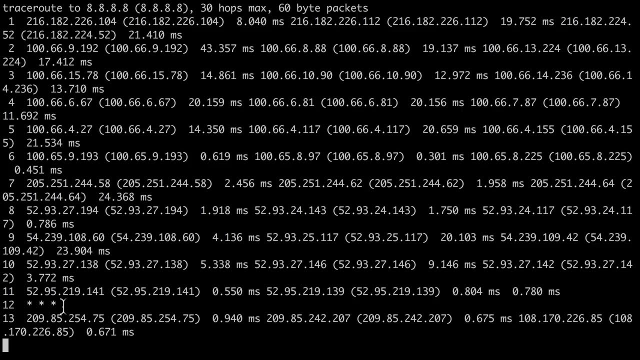 As we did before And here we can see, the traceroute command shows us the status of our network trace as it goes through multiple hops across the network. There are some hops on the network that don't respond to the traceroute command And in most cases that's okay. 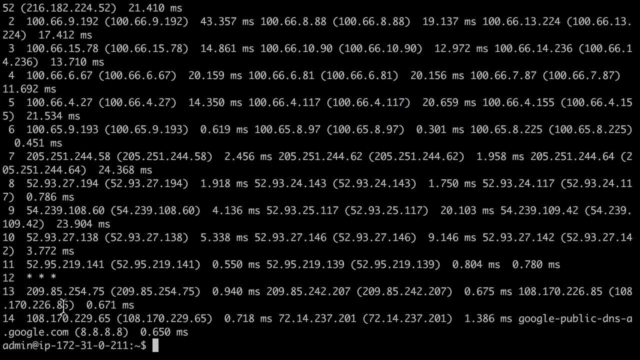 As long as you get a final response from the server that you're tracing to. In this case, we were able to do a traceroute to Google's public DNS servers. We can see that we went through 14 hops to get there And we had a really good response. 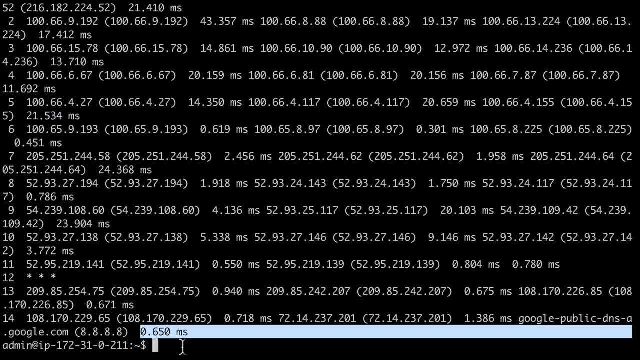 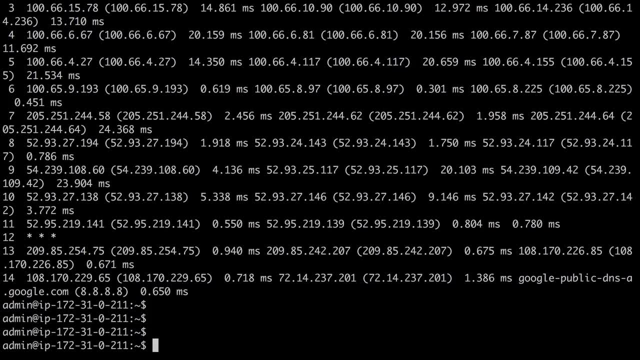 0.65 milliseconds from the final trace that we sent to the 8.8.8.8 IP address. So that's the traceroute command. You can also run these commands with DNS IP addresses to see if you have DNS resolution. 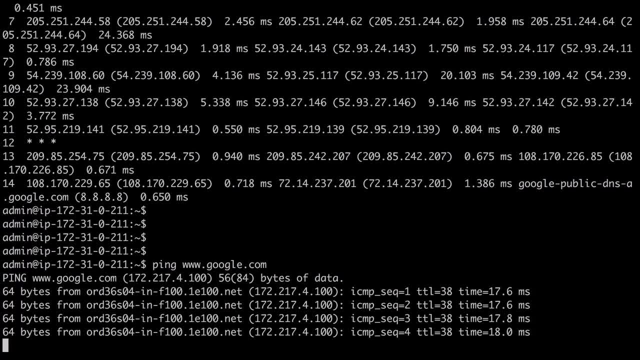 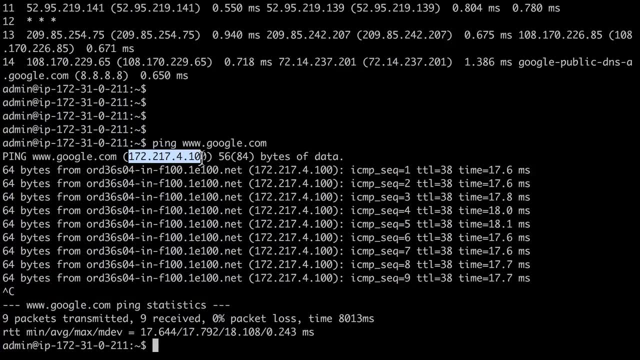 For example, here I'm pinging googlecom And you can see we were able to resolve the IP address From the DNS name, From the host name that we provided, And again we had 0% packet loss. So we do have DNS resolution working here. 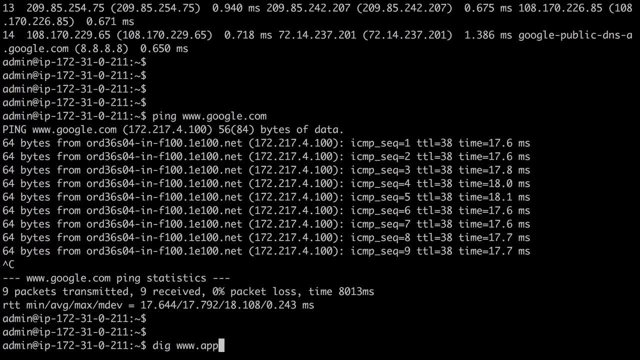 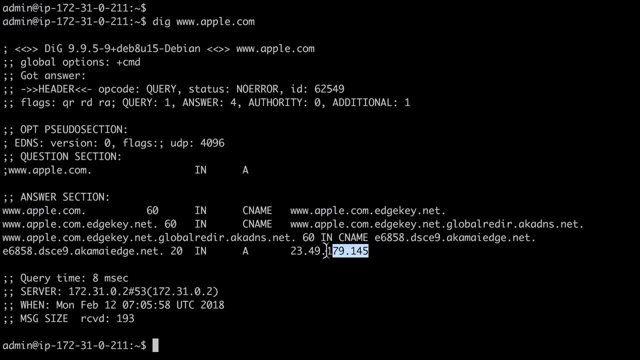 You can also use the dig command. For example, let's dig applecom And the dig command looks up a DNS record And here you can see the IP address that that DNS record should be resolving to Dig is used for DNS troubleshooting. 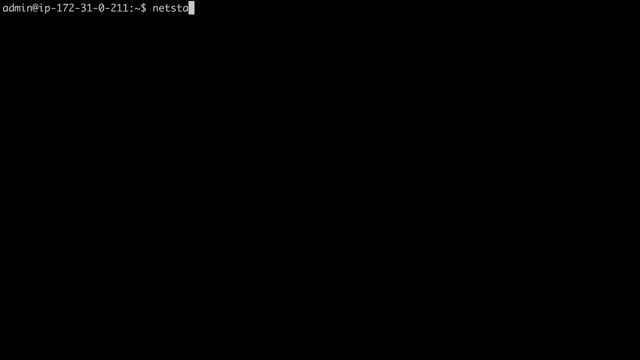 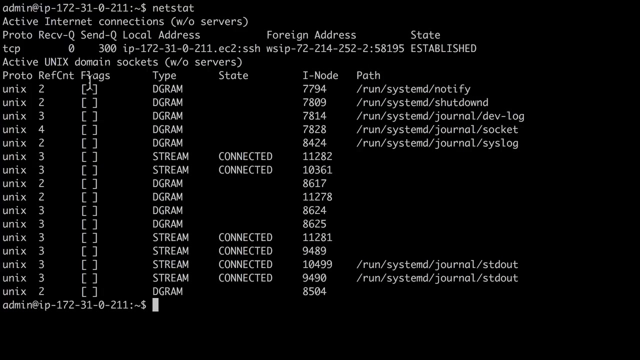 Another network troubleshooting command that I really like to use Is netstat, Which is, of course, network statistics. If you just run it by itself, It shows you the active sockets on your host And the active internet connections. For example, you can see we have an established connection. 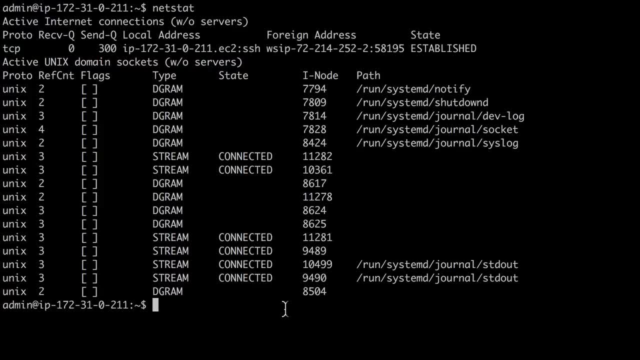 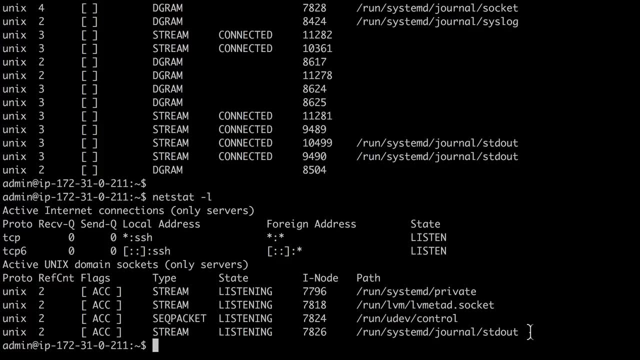 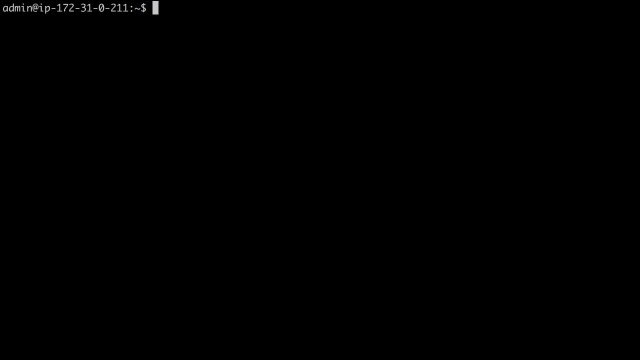 Right here to this IP address. I like also to use netstat-l To show listening connections on this host. What programs, what processes are actively listening for inbound network traffic? So, to summarize, You always need to know if your interfaces are up. 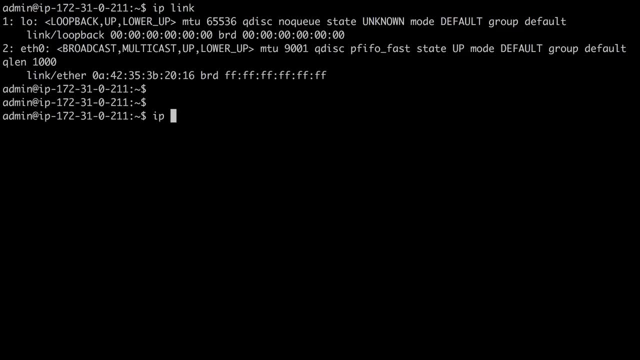 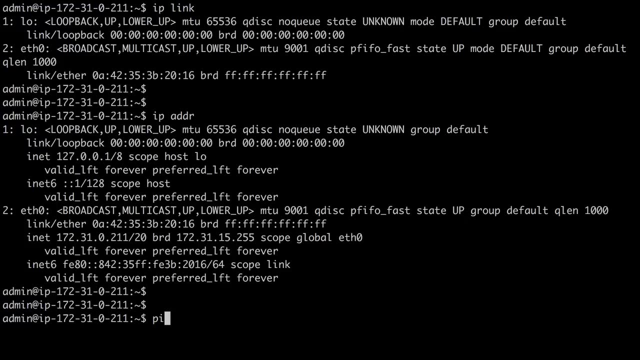 You do that with IP link. You always need to know if your interfaces have IP addressing configured. You do that with IP address. You always need to know if you have network reachability. You do that with the ping command And you can also trace the route that your network traffic takes. 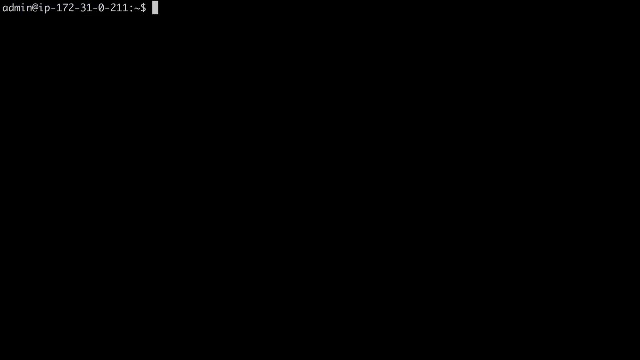 With the traceroute command. I also want to point out that the IP commands that were used in this video Are available and standard On all Linux distributions As part of the IP route 2 package, But some of the usages of these commands 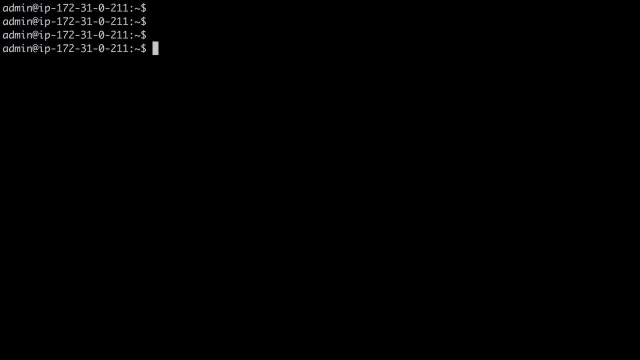 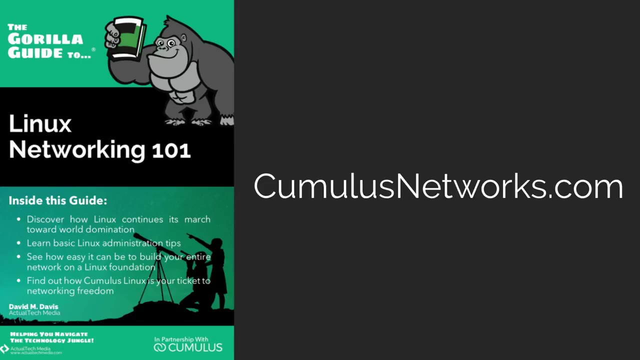 May be different from one Linux distribution to another. To learn much, much more about Linux networking, I hope that you'll check out my book, The Guerrilla Guide to Linux Networking 101.. It's available for free from cumulusnetworkscom. Thanks for watching.